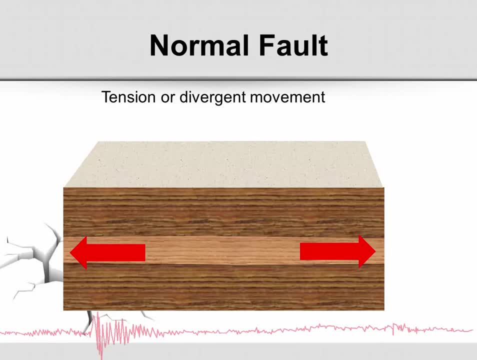 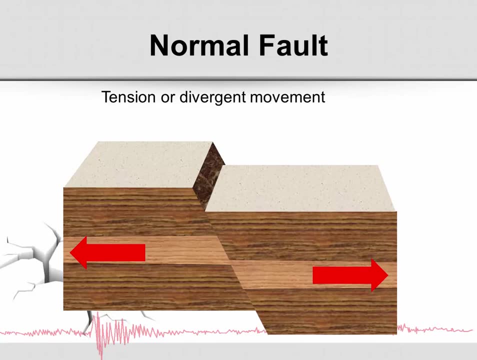 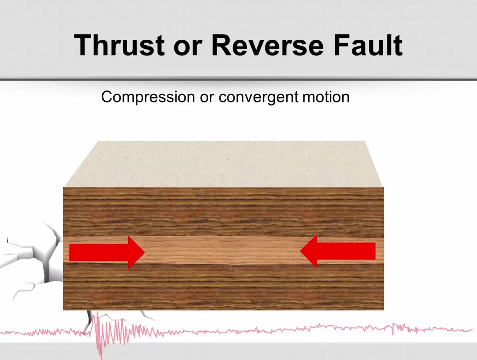 This happens with tension or divergent motion. If the rock is more rigid and less likely to stretch, it may simply crack, And when it does, one block may drop lower than the other. This is what's called a normal fault- Opposite the normal fault. we have a thrust or reverse fault. 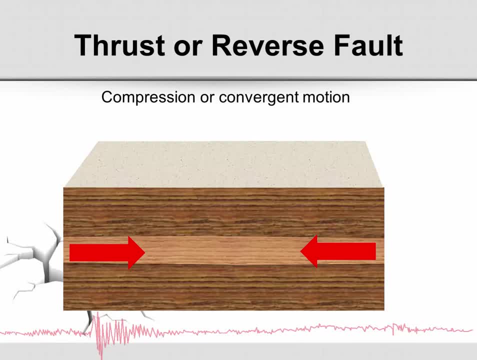 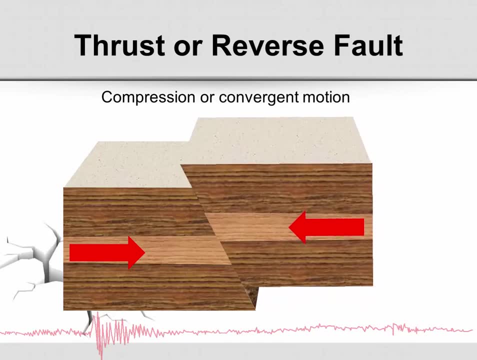 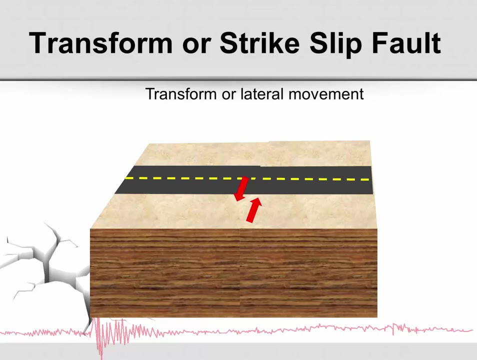 This occurs from compression or convergent motion. When two plates are pushing against each other, one plate may go down or another one may go up. This creates a thrust or reverse fault. Finally, a transform fault or a strike-slip fault occurs with lateral stress. 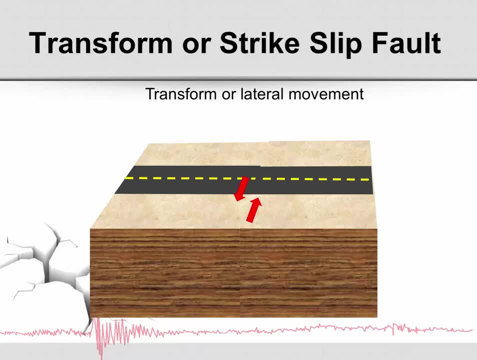 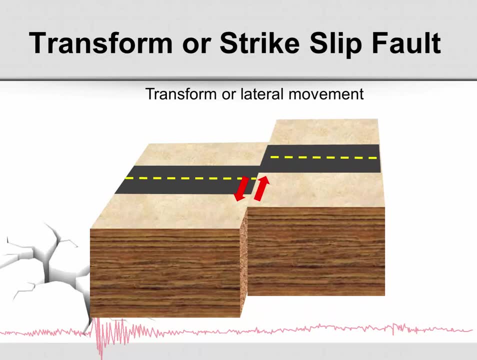 When two parts of the Earth's surface are moving in opposite directions with respect to each other, one may slide, causing a transform or a strike-slip offset. While sometimes rocks break with faults, sometimes they're soft enough to fold. A fold occurs with compression or convergent motion. 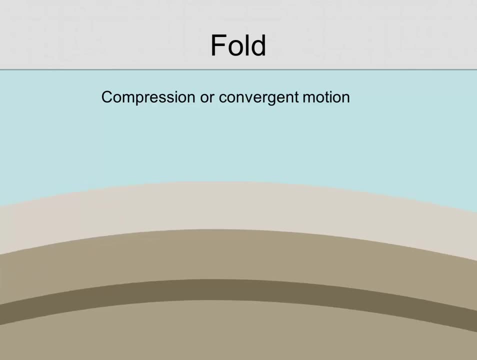 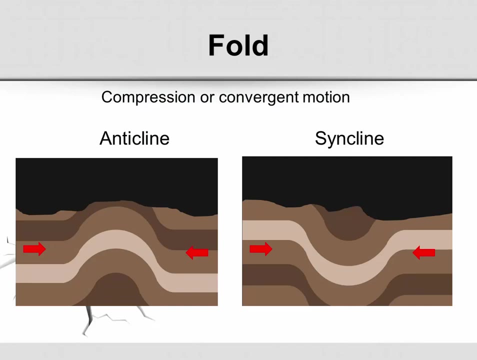 Sometimes rock layers may fold with an upward bend. Other times they may form with a downward bend. Both types of folds occur with compression or convergent motion. An up-fold is referred to as an anticline. The downward or U-shaped fold is referred to as a syncline. 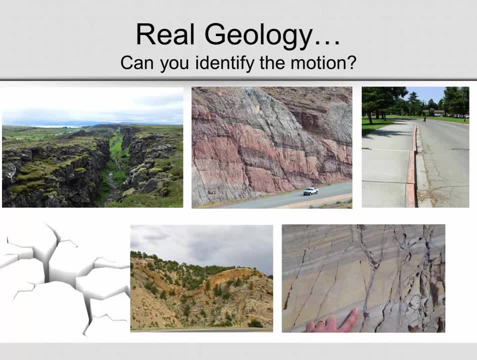 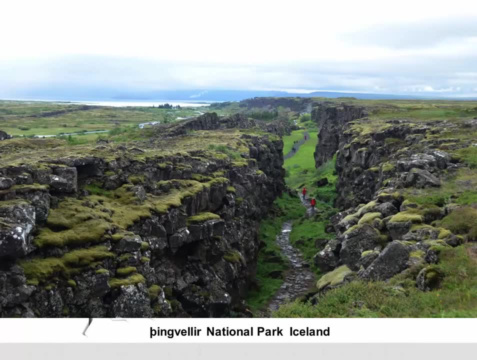 Let's take a look at what this looks like with real geology. Can you identify the motion from these real images? Let's take a look at these five different features. Thingvellir National Park in Iceland is one of the classic locations where the Earth is splitting apart. 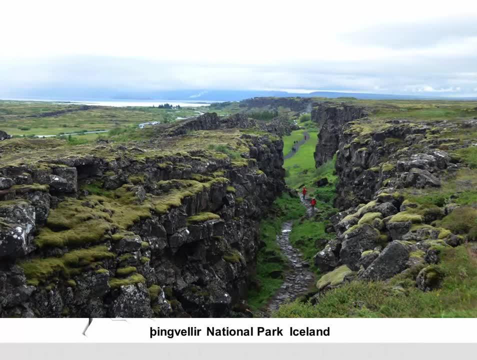 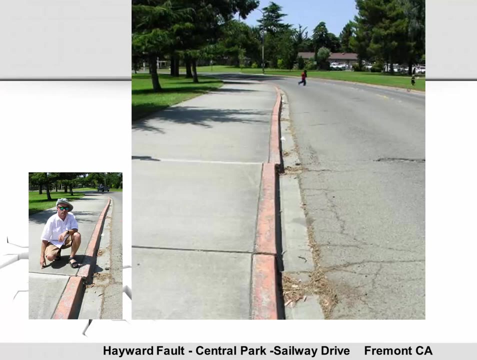 On the right-hand side of the picture we see the North American plate, On the left side the European plate. As the plates are splitting apart, this rift or gap is opening up. This occurred through divergent motion. This picture of the Hayward Fault was taken in Fremont, California, in Central Park. 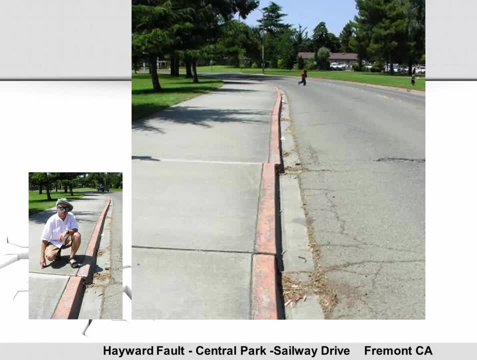 You can see, when the road planners built this road, they didn't intentionally offset the sidewalk and curving. What happened here is part of the road was built on the North American plate and the other part of the road was built on the Pacific plate. 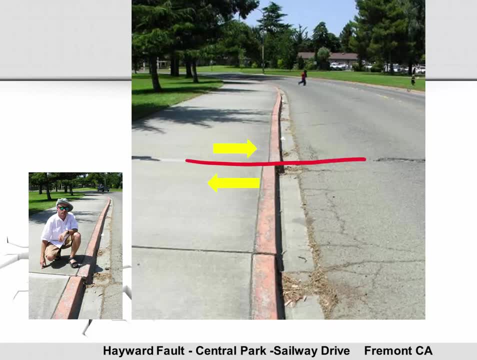 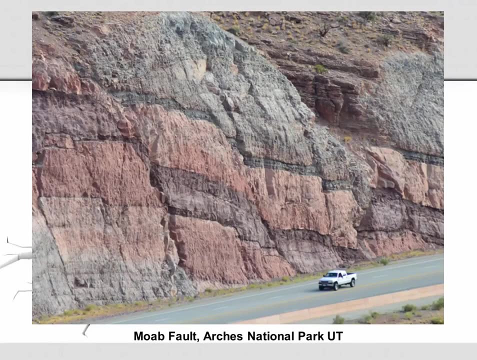 Here's the fault line and we can see the further section is moving northward, where the side that the photographer is standing on is moving towards the south. Moab Fault is a dramatic fault that was revealed in a road cut just outside of Arches National Park in Utah. 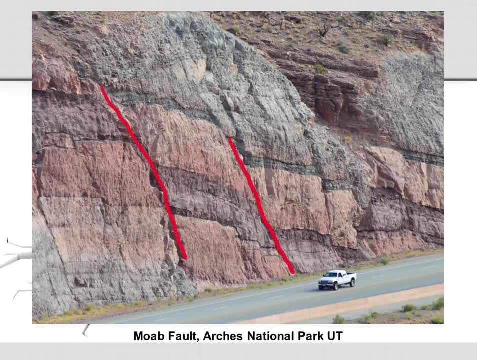 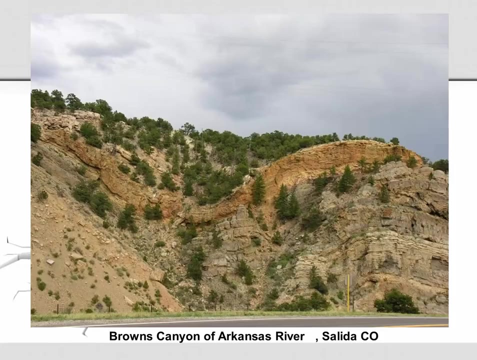 Here we can see several very large faults. As we identify the previously aligned layers, we can see that this brown stripe used to all be the same layer but now has been offset with several normal faults. This represents divergent motion or tension. Browns Canyon of the Arkansas River goes through Salida, Colorado. 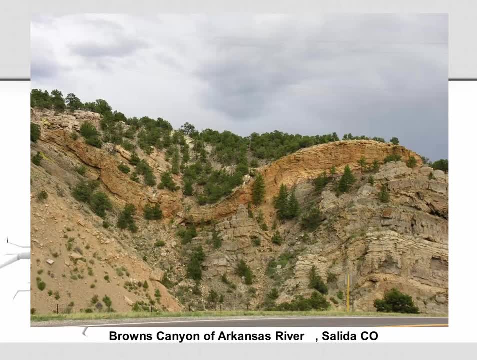 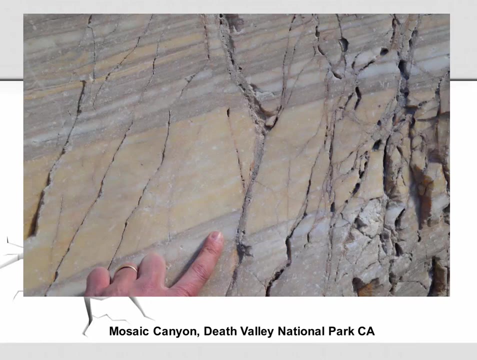 Here we can see rock layers that have been folded. This must have occurred through compression or convergent motion. It's impossible to make a fold by pulling, Going from a large scale to a rather small scale. in Mosaic Canyon in Death Valley National Park, California. 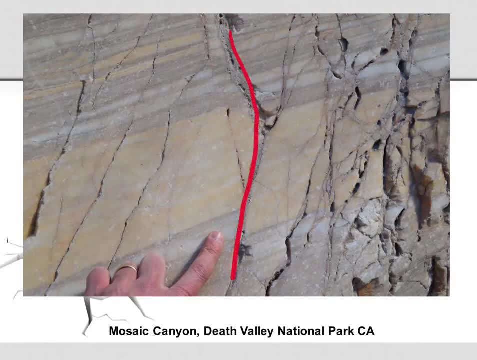 we can see this small layer was offset, The fault indicated in red and these yellow layers are offset with a little bit of overlap. This indicates that this was a reverse fault caused from compression or convergent motion. So let's take a little quiz. 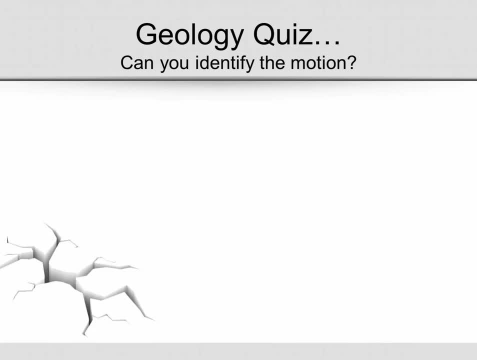 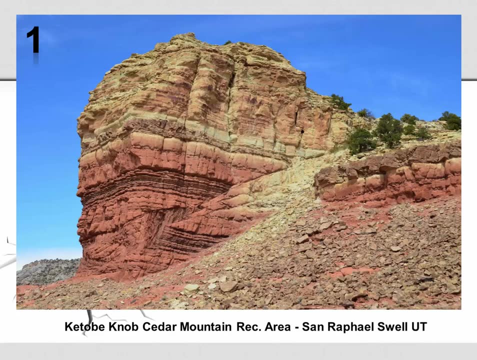 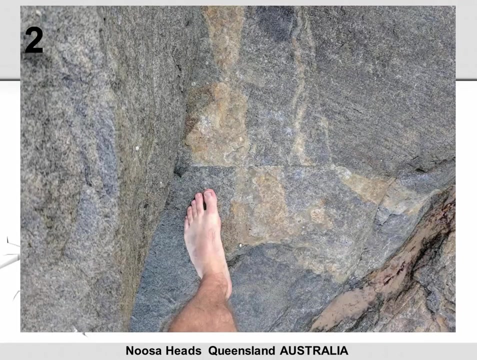 Can you identify the motion in these next five images? Feel free to pause the video between each image. Number one is Katobi Knob, located in the Cedar Mountain Recreation Area in the San Rafael Swell in Utah. Number two is a rock structure that I found at Noosa Heads in Queensland, Australia. 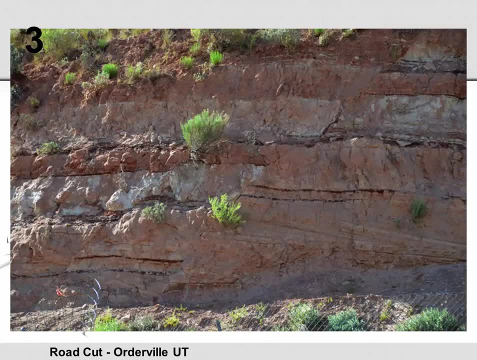 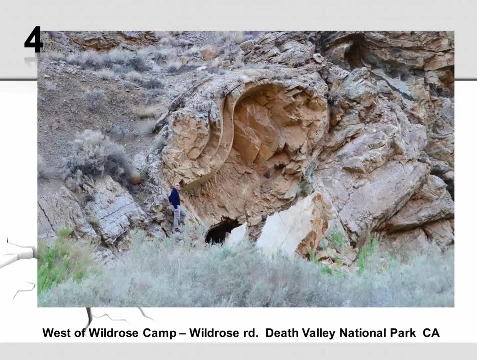 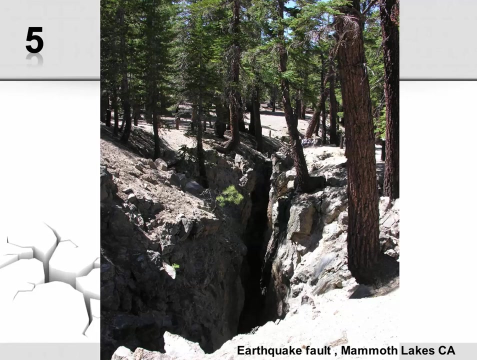 Number three, a road cut near Orderville, Utah. Number four: rock layers west of Wildrose Campground on Wildrose Road in Death Valley National Park. Number five is specifically called Earthquake Fault, located just outside Mammoth Mountain Ski Area in Mammoth Lakes, California. 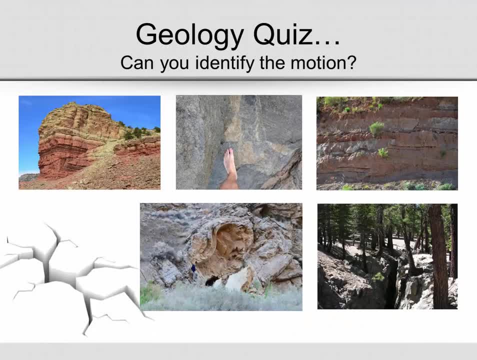 So could you identify all five of these images? What sort of plate motion caused each? Are they normal faults, reverse faults, folds or rifts? Let's take a look at each Number one: Katobi Knob in the San Rafael Swell in Utah.